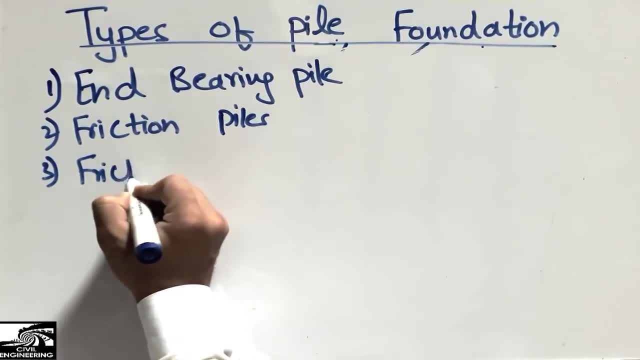 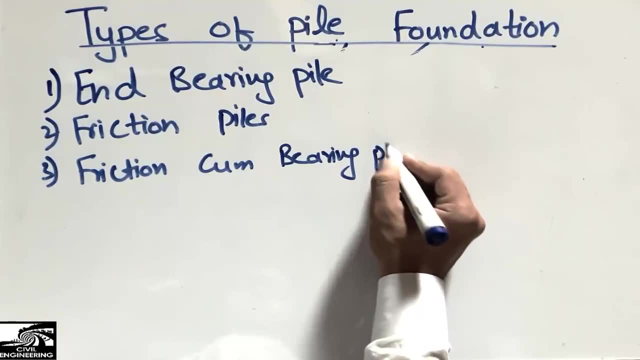 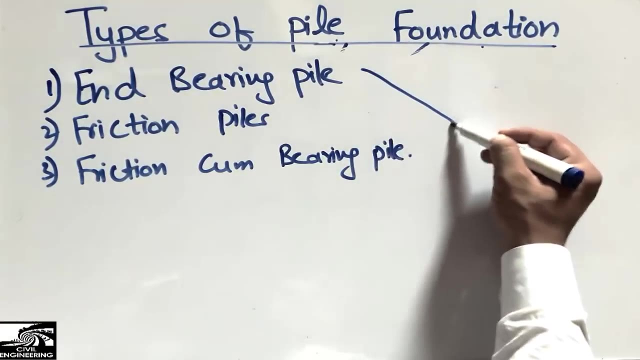 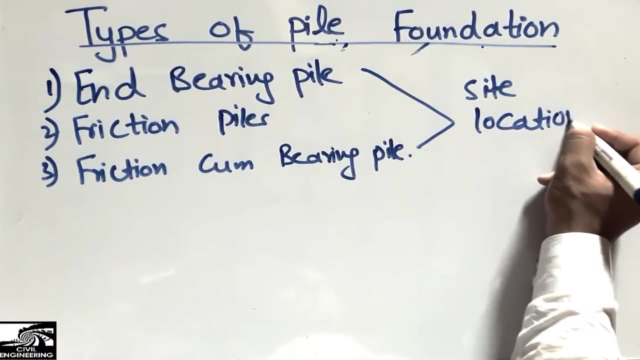 The third one is the friction cum bearing pile: Friction cum bearing pile. So there are three main types of the pile, depending on the location. Depending on the site location, We use these types of the pile depending on the site location, Whether your foundation soil is hard or soft. 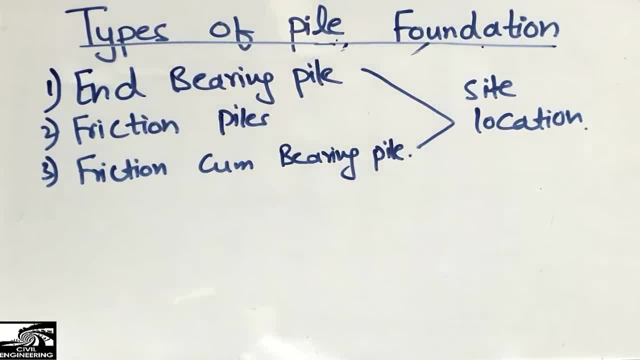 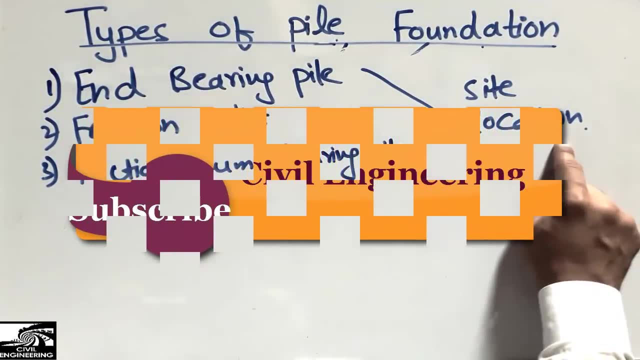 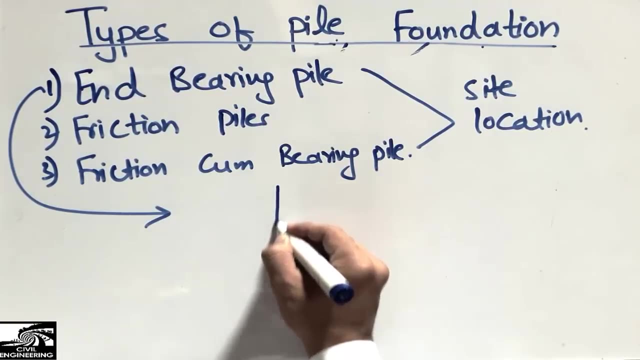 So we use these three different types of the pile And the engineers decide these three different types of the pile Depending on the site location. So to define the first one is the in-bearing pile. In-bearing pile- This is the pile We do the pilings. 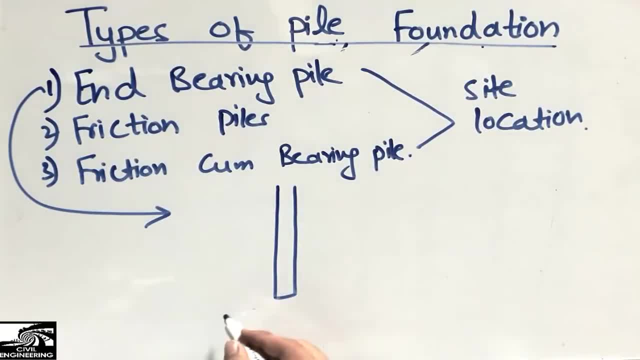 And in-bearing pile is the type of the pile foundation which is based on the hard state of the soil. This is the hard rock, Hard state or the hard rock. So the foundation, which is the piling which we do on the hard rock. 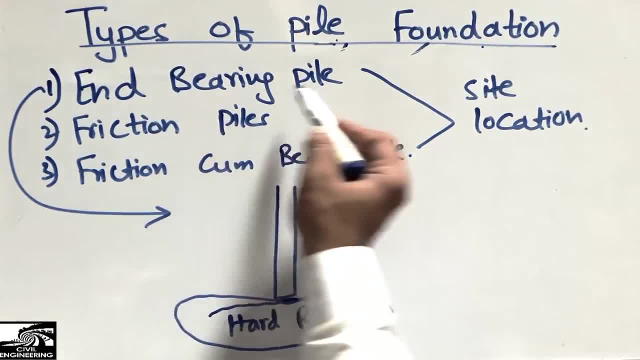 We call it the in-bearing pile Because the load coming on this pile now will be taken by the rock. The whole resistance will be provided by the rock in the upper direction. So this rock is hard. state of the soil is able to support this load. 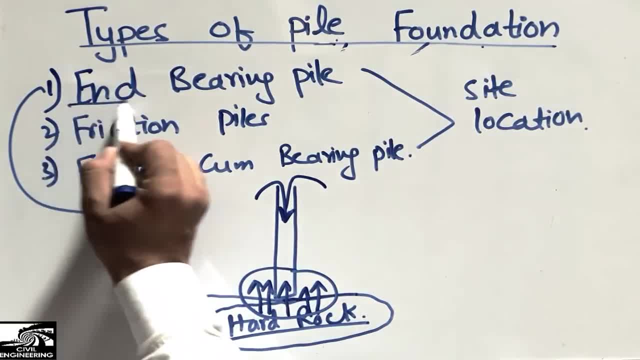 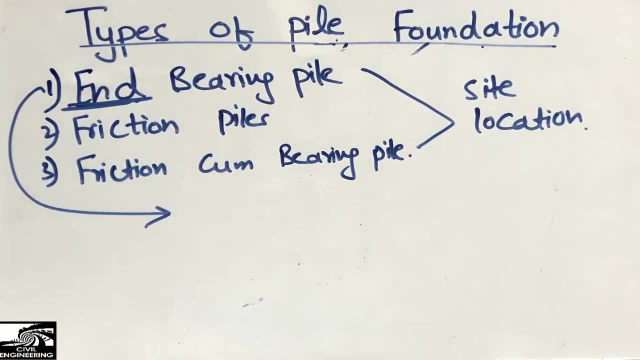 So we call it the in-bearing pile, Because the load is coming on the end of the pile. Now coming to another type of the pile: The friction piles. The friction piles are those piles where the hard rock, state of the here, the state of the soil, 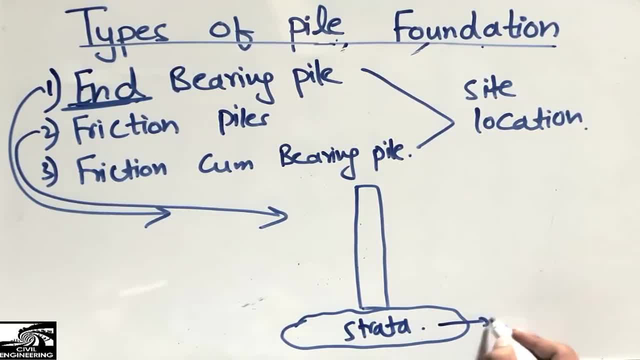 The soil state of the soil is weak, Is weak. So what we do, We do. the piles that are the whole resistance to this load of the pile, To this load of the pile, is provided by the friction of the piles. Mainly there is the whole resistance is offered to these loads by the sides of the pile. 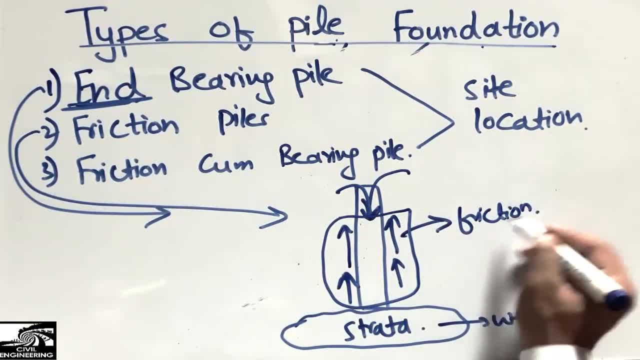 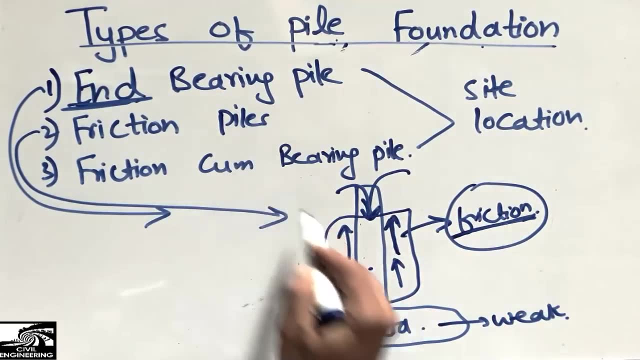 So we call this type of the pile is the friction piles, Because the whole resistance to this load is provided by the side of the pile. By which method? By the friction method to the upcoming load on the pile. So we call this type of the pile is the friction pile. 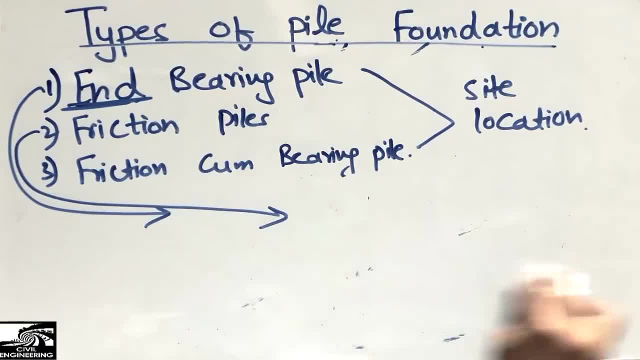 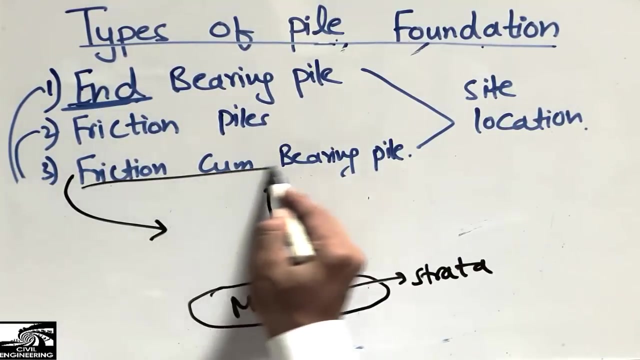 Now the third type of the pile is the friction cum-bearing pile. It is the type of the pile In which the strata is normal, is medium, And with this strata And also So this type- this is the type of this- is the combination of these about two piles. 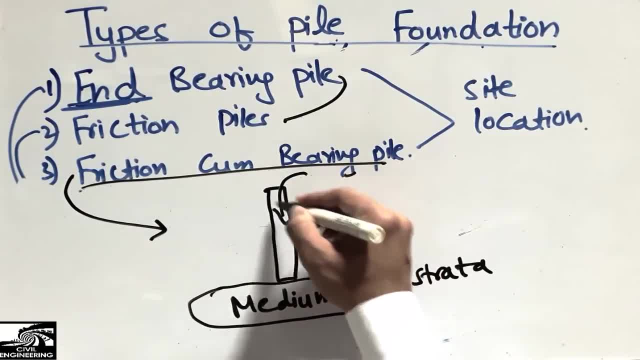 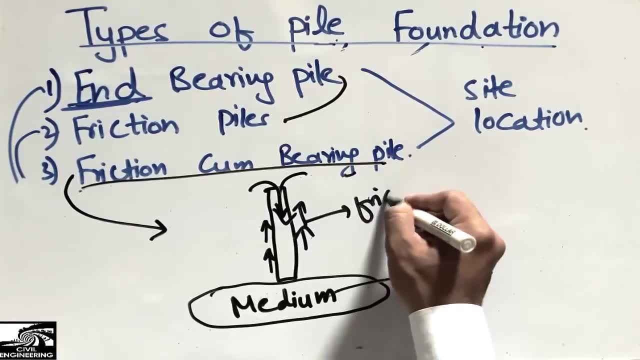 Friction, cum-bearing piles, It is also provided. This is the load, for example, coming on the pile. So the sum of the resistance is provided by the friction, By the method of friction, And the sum of the resistance is provided by the in-bearing pile. 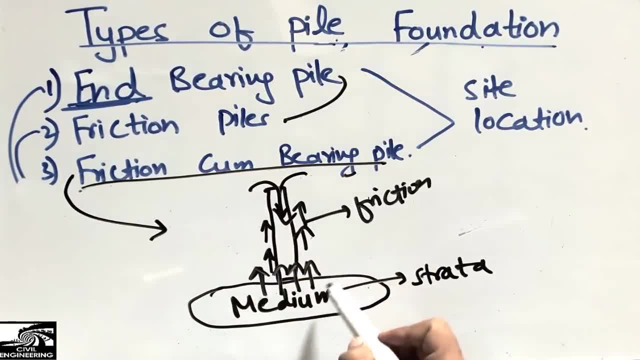 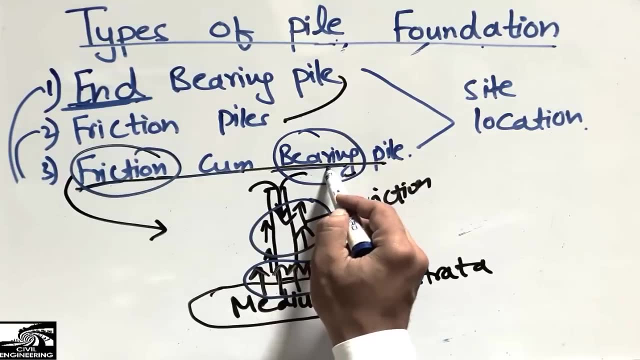 It means that the both actions are included in this type of pile: The in-bearing as well as the friction pile. So this why its name is friction cum-bearing pile: The friction phenomena as well as the in-bearing phenomena. So this type of pile we call as the friction cum-bearing pile. 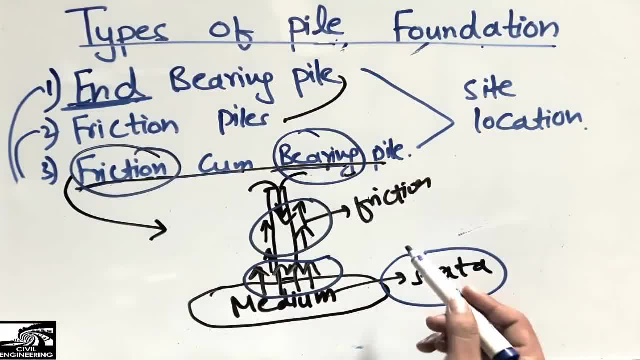 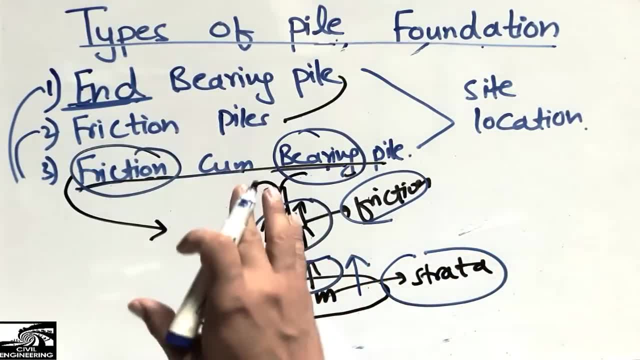 And this type of pile, the strata is medium. So what we do, We provide the sum resistance by the in-strata And the sum resistance by the friction. These were the three main types of the pile. foundation were used And we select this type of foundation depending on the site location. 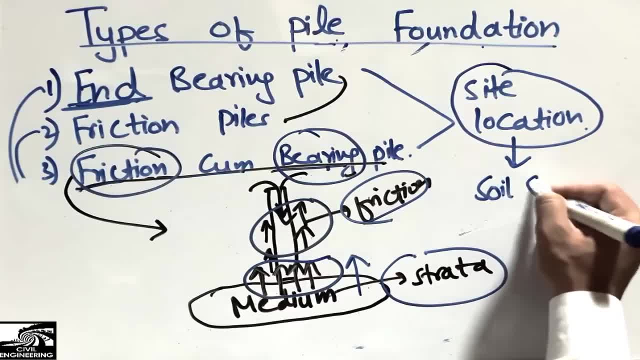 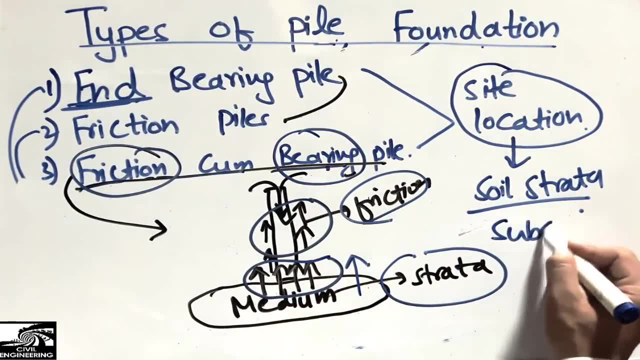 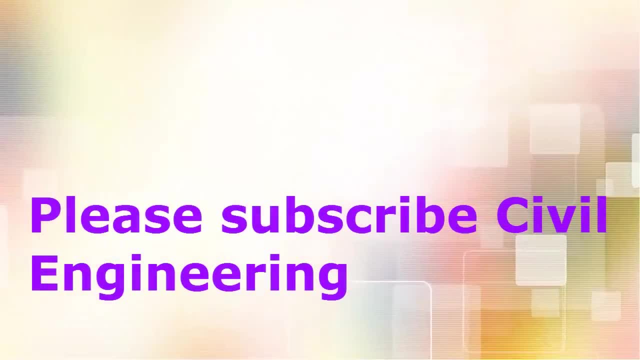 Depending on the soil strata, Which type of soil strata we are using. And don't forget to subscribe our channel for other civil engineering videos. Thank you for watching our video. Thank you for watching our video.